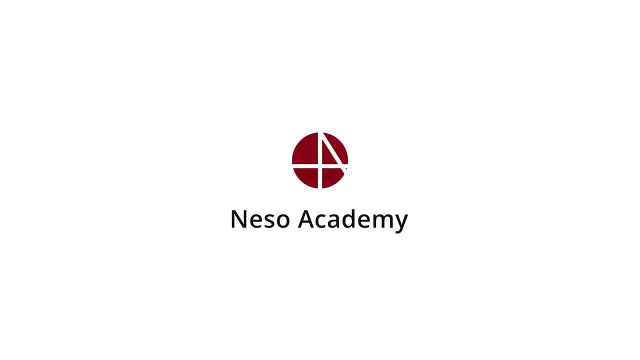 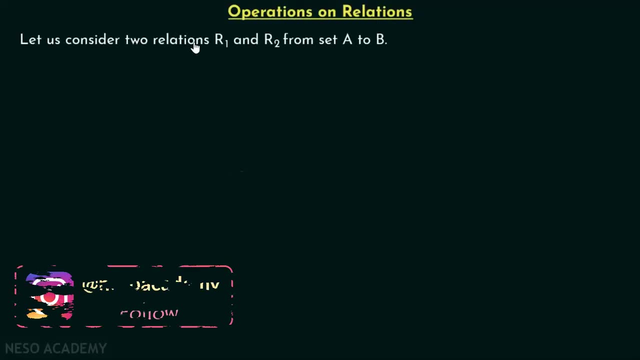 Now we will discuss some operations on relations. Let us consider two relations, R1 and R2, from set A to set B. These relations can be combined in a way, two sets can be combined, That is, R1- union, R2, R1 intersection, R2, R1 minus R2, R2 minus R1. 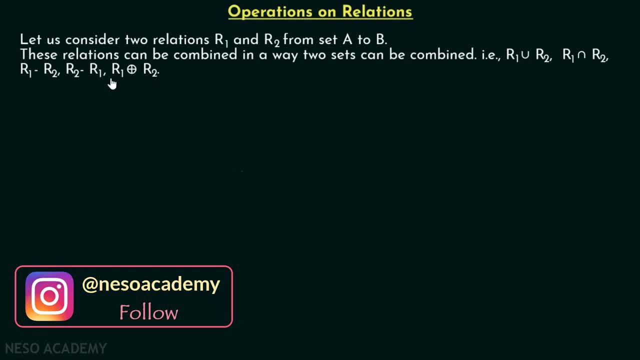 and symmetric difference of R1 and R2.. These are all the possible operations which we can perform on relations. okay, Obviously, these operations we have already seen in case of sets right, But in relations also we can apply these operations like union intersection difference and symmetric difference. okay. 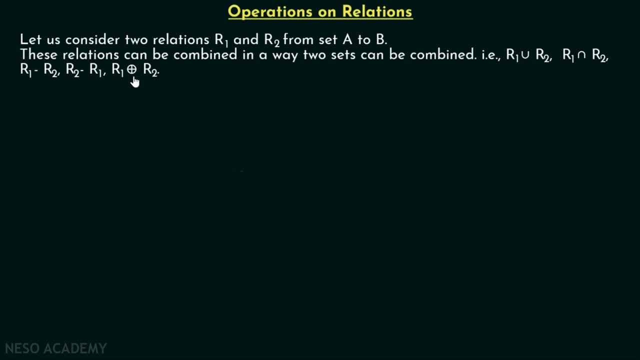 Now let us discuss one example which helps us in understanding how do we able to combine two relations by using these operations. okay, Let us say we have a set A which consist of three elements- 1,, 2, 3- and we have a set B which consist of three elements. 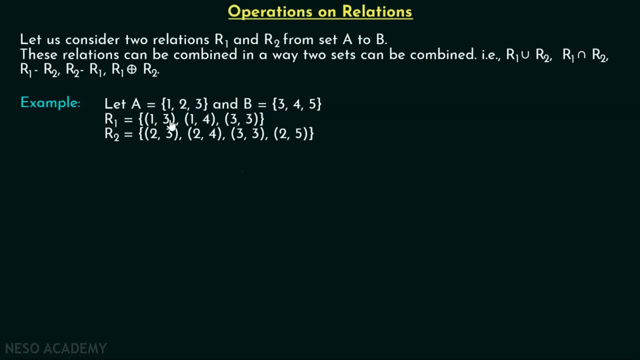 3, 4, 5.. R1 is a relation which consist of these ordered pairs: 1, 3,, 1, 4, 3, 3 and. R2 is a relation which consist of these ordered pairs: 2, 3,, 2, 4, 3, 3, 2, 5.. 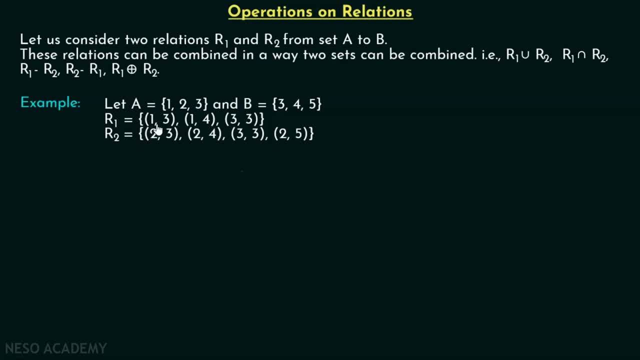 Now, what is R1, union R2?? It must contain every ordered pair of R1 and every ordered pair of R2.. And this is how it looks like: 1, 3, 1, 4, 2, 3, 2, 4, 2, 5, 3, 3.. 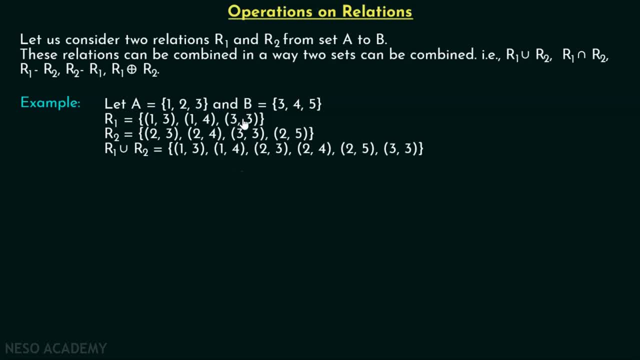 Here. obviously, 3, 3 is repeated, right. 3, 3 is there in R1 as well as R2.. We must write it once in: R1- union- R2, right? So this is R1- union- R2, which consist of these ordered pairs. 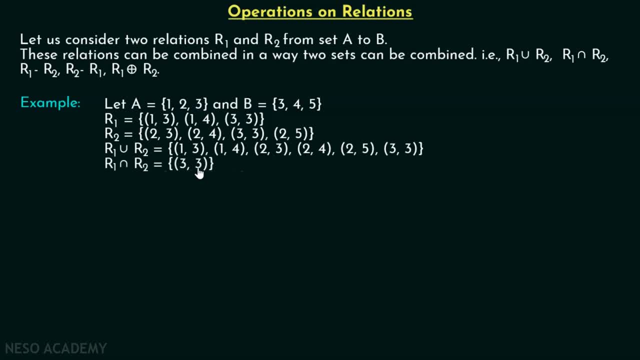 Now, what is R1 intersection R2?? Obviously, this is this ordered pair only right 3, 3, because this is the only ordered pair which is common between R1 and R2.. Now what is R1 minus R2? R1 minus R2 must include every element of R1. 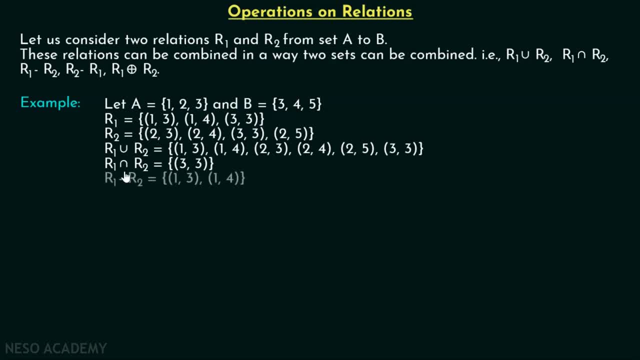 but it must not include any element of R2, right. So R1 minus R2 must consist of these ordered pairs: 1, 3, 1, 4, right: 1, 3, 1, 4.. 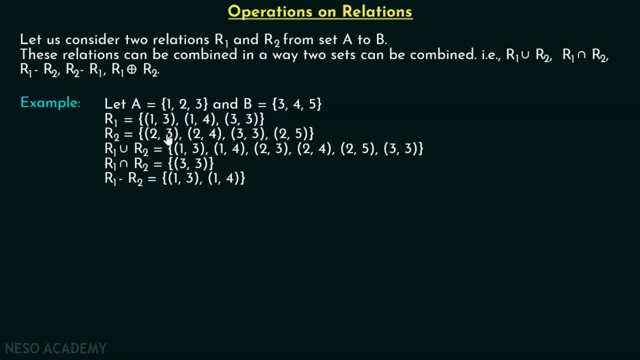 3, 3 must not be there in R1 minus R2, because 3, 3 is there in R2, right. Now, what is R2 minus R1?? Again, every element of R2, but no element of R1, right. 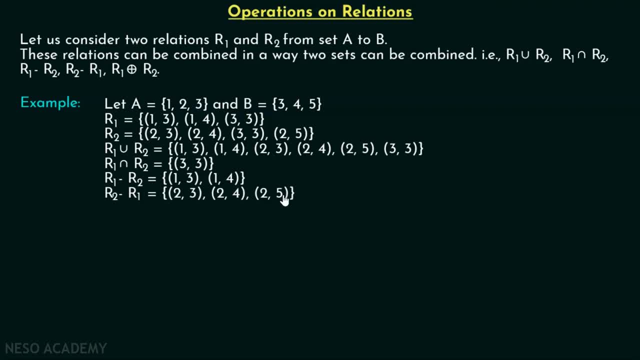 2,, 3,, 2,, 4, 2, 5.. Now, what is symmetric difference of R1 and R2?? Symmetric difference of R1 and R2 is actually equal to R1- union R2 minus R1, intersection R2.. 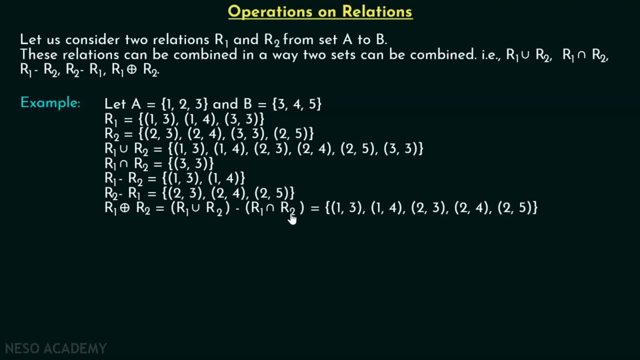 We already know this right. This is from the definition of symmetric difference. Symmetric difference of R1 and R2 is actually equal to R1 union R2 minus R1 intersection R2.. R1 union R2 minus R1 intersection R2.. 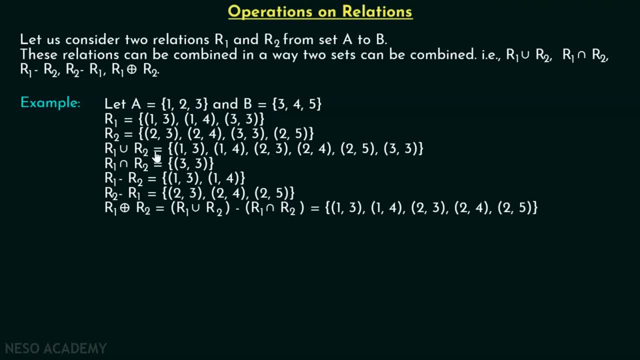 This means every element of R1, union R2, but no element of R1 intersection, R2, right. This means 1, 3, 1, 4, 2, 3, 2, 4, 2, 5. 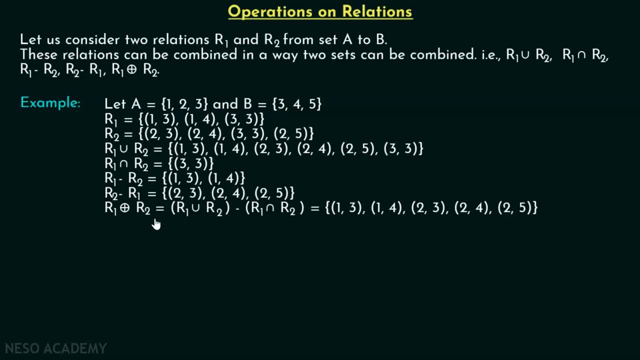 must be included in symmetric difference of R1 and R2.. 3, 3 must not be included, because 3, 3 is there in R1 intersection R2, right, So it is clear that symmetric difference of R1 and R2. 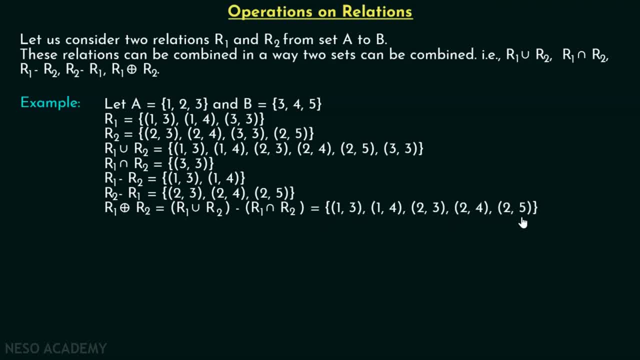 consists of R1 and R2.. It consists of these ordered pairs: 1, 3, 1, 4, 2, 3, 2, 4, 2, 5,. right Now we will discuss one problem related to operations on relations. okay. 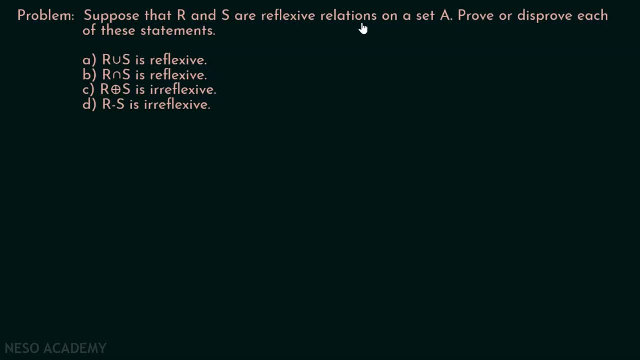 Let's discuss this problem. Suppose that R and S are reflexive relations on a set A. okay, These two are reflexive relations and they are defined on set A. Prove or disprove each of these statements: R union S is reflexive. 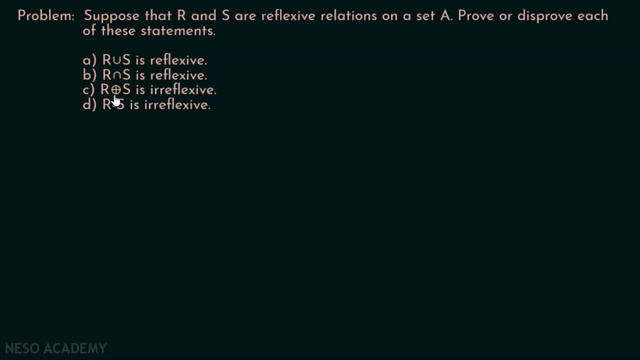 R intersection S is reflexive. Symmetric difference of R and S is equal to R1 and R2.. R is irreflexive. R minus S is irreflexive. okay, Let's consider this option first, that is, R union. S is reflexive. 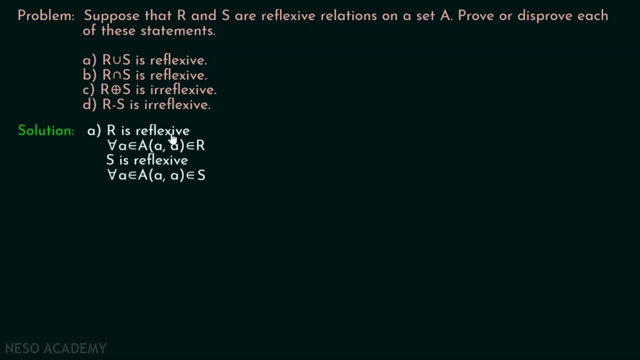 We are given with this information that R is reflexive. Now we know that if R is reflexive, then for every element A belong to A. A comma A must belong to R, And if S is reflexive, then for all element A belong to A. 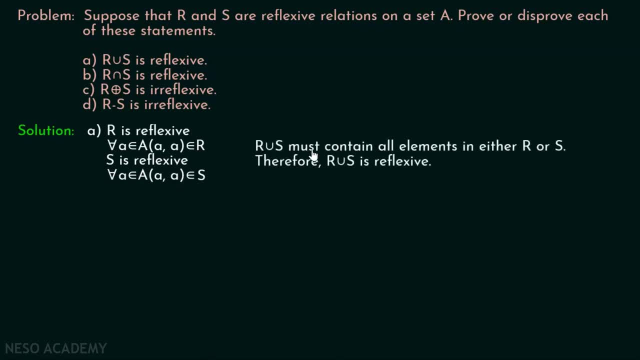 A. comma A must belong to S. Now you know that R union S must contain all elements in either R or S Right. This means that every element of R and every element of S must be included. So it is clear from this fact that R union S is reflexive. 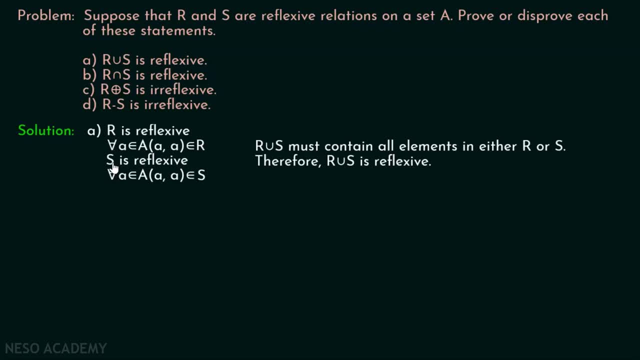 Because R is reflexive and S is reflexive. Right Now, let's consider option B: R intersection S is reflexive. We know that R is reflexive, right? This means for every element A belong to A, A comma A must belong to R. 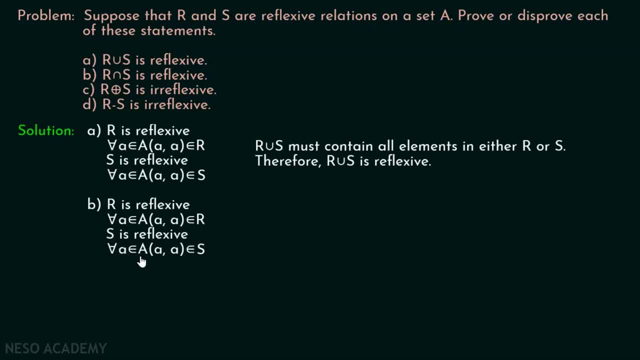 And we know that S is reflexive, which means for all element A belong to A, A comma A must belong to S, R intersection, S must contain all elements in both R and S, And we know that R is reflexive and S is also reflexive. 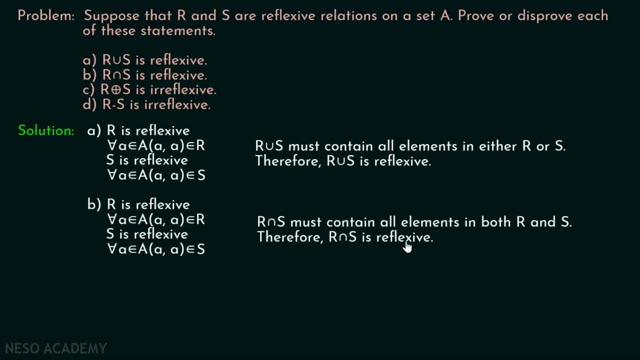 Therefore, R intersection S must be reflexive, Right? So this is also clear. Let's consider this option. Symmetric difference of R and S is irreflexive. We know that R is reflexive and S is also reflexive. 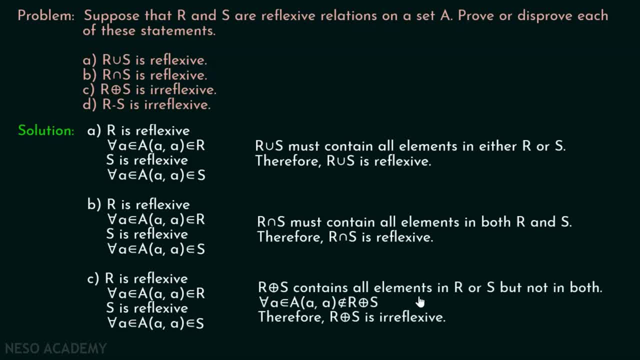 Symmetric difference of R and S contains all elements in R or S, but not in both Right, Which means for all element A belong to A A comma A does not belong to symmetric difference of R and S Right. We are talking about symmetric difference of R and S. 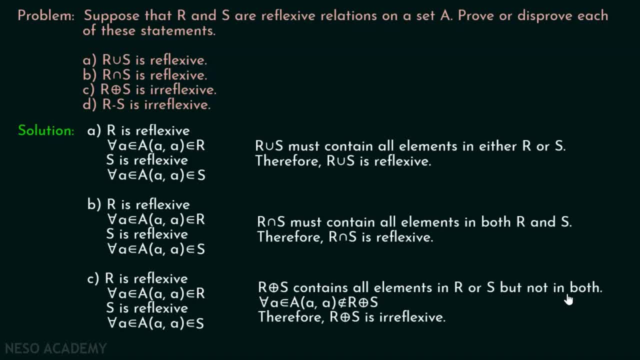 It must contain all elements in R or S, but not in both. So it is clear that for all element A belong to A comma. A must does not belong to symmetric difference of R and S. Therefore it is clear that symmetric difference of R and S is irreflexive. 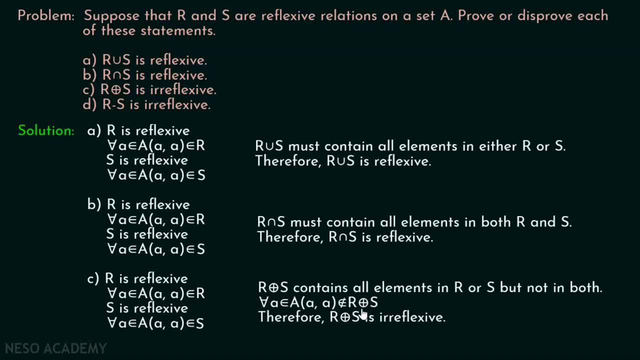 Isn't that so? This does not belong to symmetric difference of R and S, Correct? Okay, Let's discuss option D. R minus S is irreflexive. We know that R and S are reflexive. R minus S contains all elements in R. 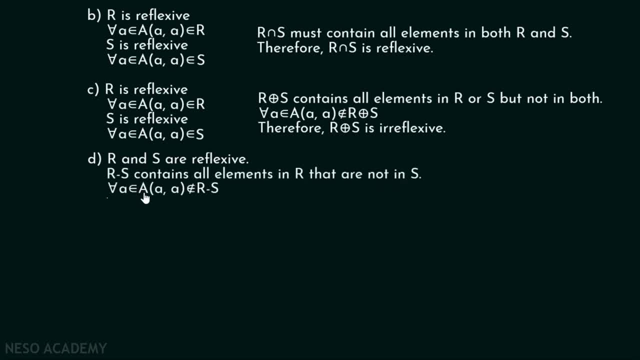 that are not in S. So it is clear that for all A belong to A, A comma A does not belong to R minus S, Because R and S are both reflexive Right. Therefore R minus S is irreflexive. 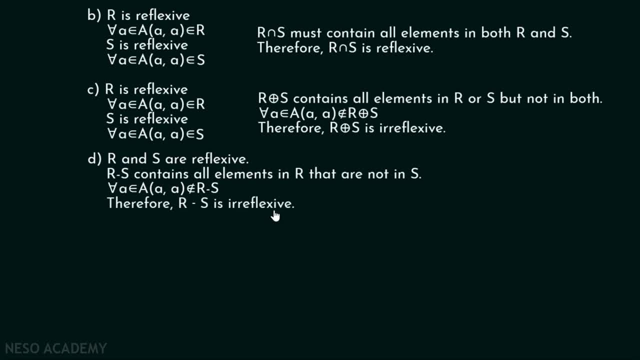 Isn't that? so Let's consider one example which helps us in cementing the concept which we have seen. Let us say that we have a set A which consists of these elements. We have a relation R which consists of these ordered pairs: 1, 1, 2, 2, 3, 3, 3, 4.. 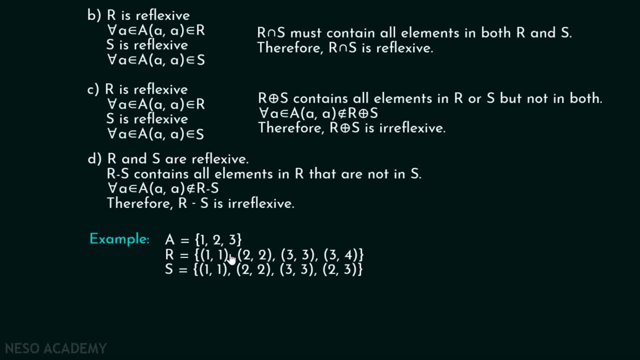 Because we know that this relation is reflexive, Therefore 1, 1,, 2,, 2 and 3, 3 must be included Right. And we also know that relation S is also reflexive, Therefore 1, 1,, 2, 2 and 3, 3 must be included. 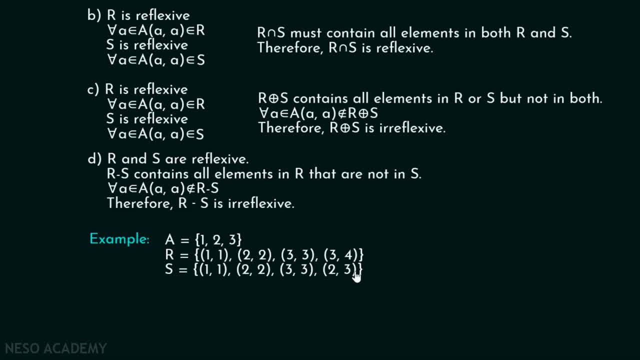 in relation S as well. Apart from this, I have included this extra ordered pair that is 2, 3.. This is some arbitrary ordered pair. Okay, R union S gives 1, 1, 2, 2, 3, 3, 2, 3, 3, 4.. 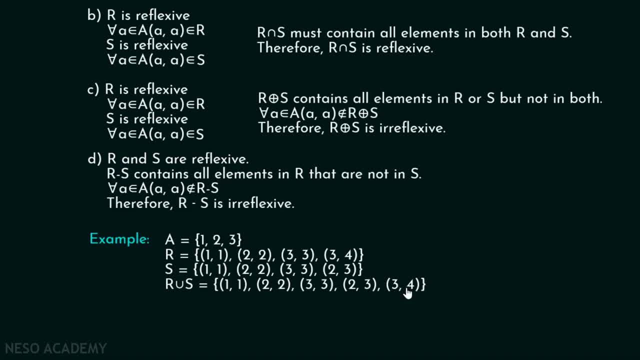 You can see that this relation is reflexive, Isn't that so? Because we are considering all elements of R and all elements of S. So definitely, 1, 1, 2, 2 and 3, 3 must be included. 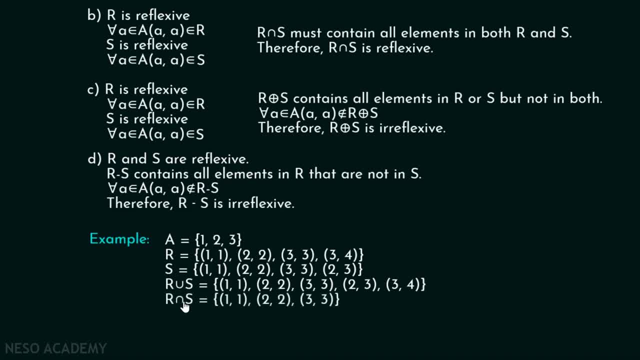 in R union S. What about R intersection S? 1, 1, 2,, 2, 3, 3.. These three ordered pairs are included in R intersection S. They are always common in between R and S Because they both are reflexive. 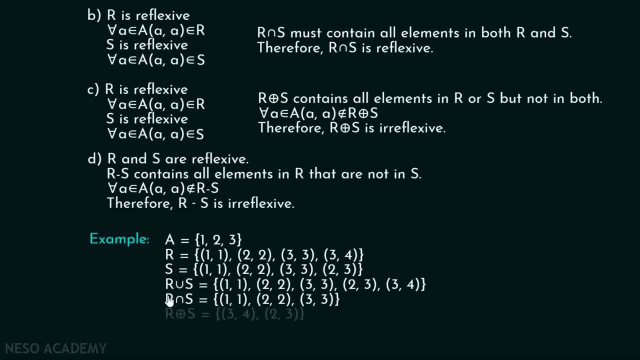 Right, Therefore R intersection S is also reflexive. What is symmetric difference of R and S? It gives 3,, 4,, 2, 3.. Right, And you can clearly see. this relation is irreflexive. There is not even a single ordered pair. 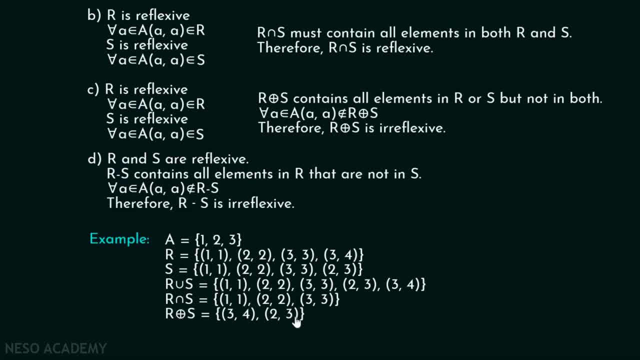 out of these ordered pairs: 1,, 1,, 2,, 2,, 3,, 3.. So it is clear that this relation is irreflexive. What about R minus S? R minus S must include every element of R. 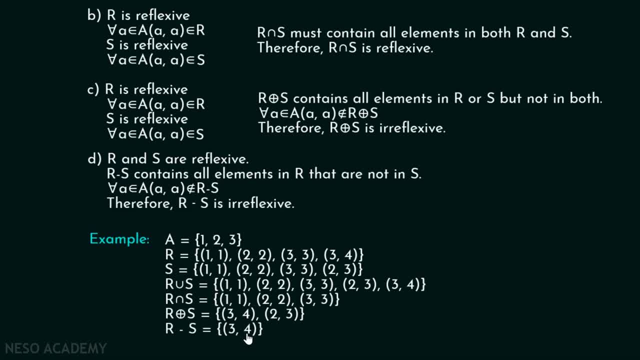 and no element of S. You can see that only 3, 4 is included in R minus S. This is irreflexive, Isn't that? so Only 3, 4 is included, So it is clear that R union S. 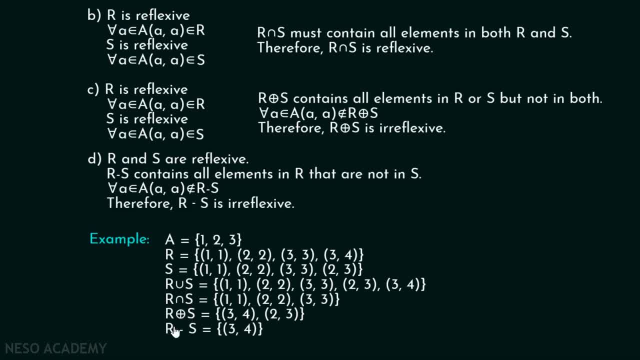 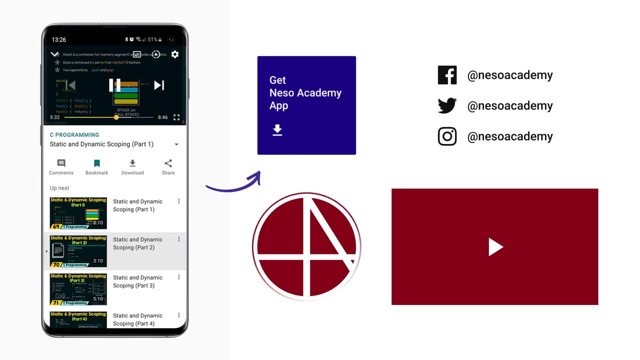 and R intersection S are reflexive relations, While symmetric difference of R and S and R minus S are irreflexive relations. Okay, Okay, friends. this is it for now. Thank you for watching this presentation. See you next time.